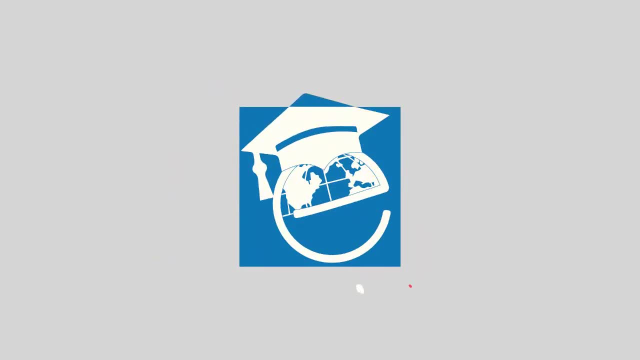 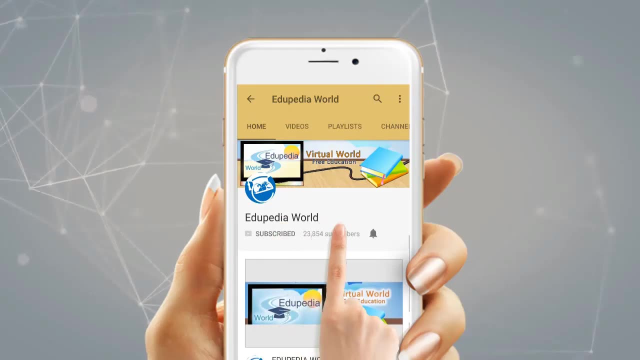 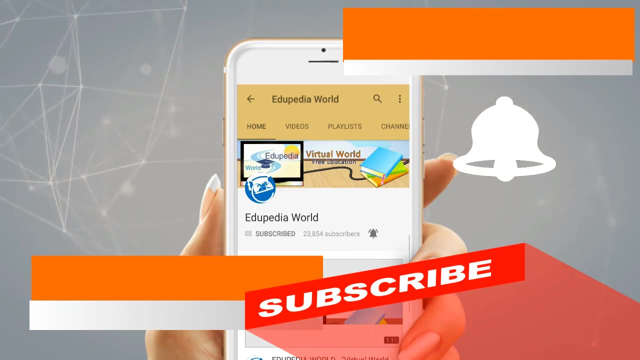 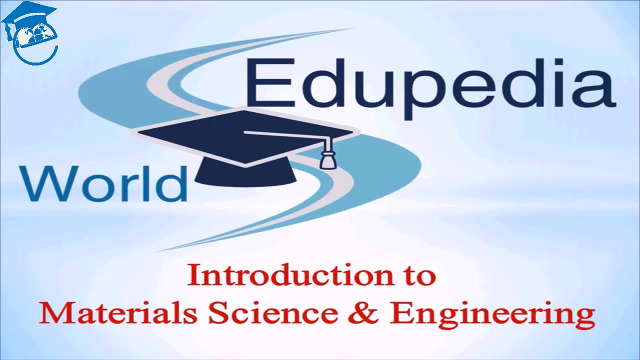 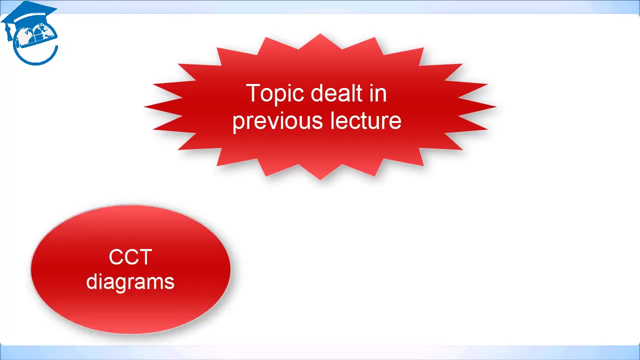 Hi everyone, welcome back to the course on Introduction to Material Science and Engineering offered by Edupedia World. Previous lecture, I introduced you to the concept of CCT curves- continuous cooling curves- and I briefly concluded a lecture mentioning about martensite. Today we will see details about martensitic transformation and what is martensite. 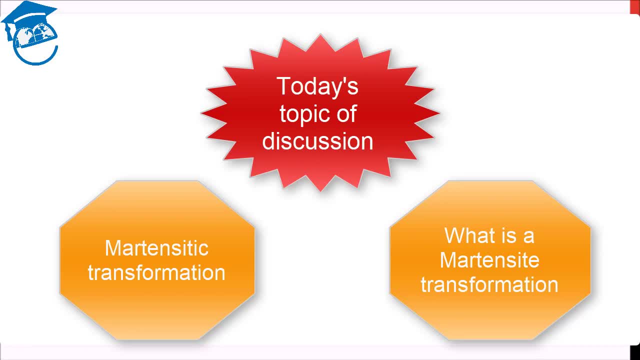 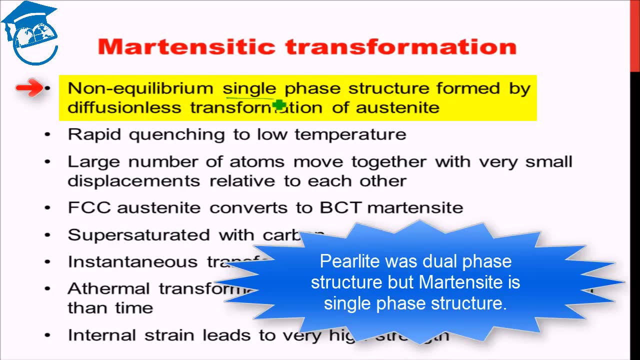 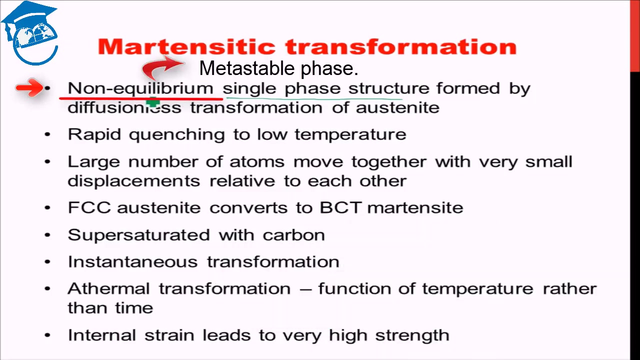 To start with, martensite is a non-equilibrium, single phase structure. Perlite was a dual phase structure but martensite is a single phase structure, but it is a non-equilibrium phase, that is, it is a metastable phase. It is not the phase where which is energetically most stable. 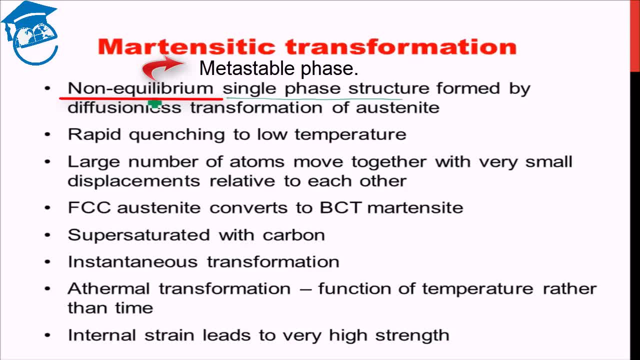 but it is the most stable. it is the phase which is present because of the kinetic hindrance And martensite is formed by diffusionless transformation of austenite. For the formation of bainite and perlite, you saw that there has to be diffusion taking place but martensitic formation. 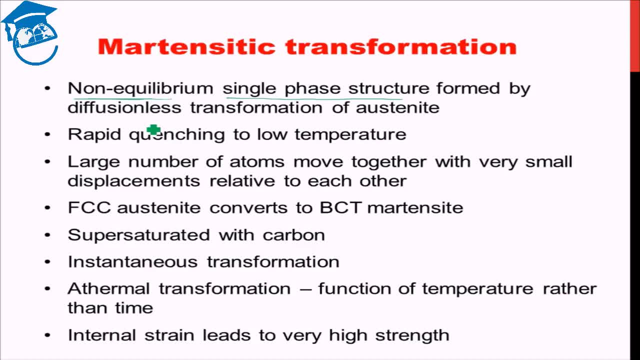 is a diffusion-less process. Diffusion is not involved during martensitic formation. How is martensite formed? Martensite is formed by rapid quenching to low temperature. You cool austenite which is at high temperature, austenitic material at high temperature. 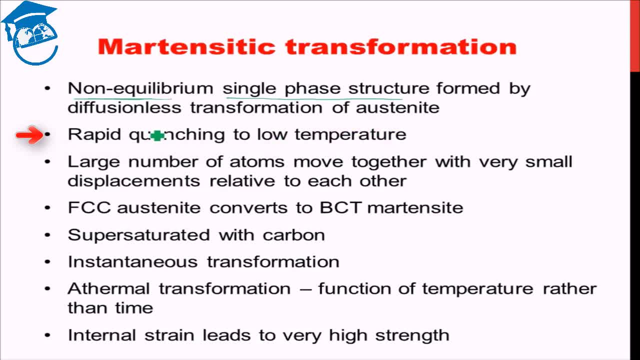 to quite low temperature, at a rapid pace that will lead to conversion of austenite to martensite. What exactly is happening during martensitic transformation? During martensitic transformation, large number of atoms, all of them, move together, and they move by very small displacement, which? 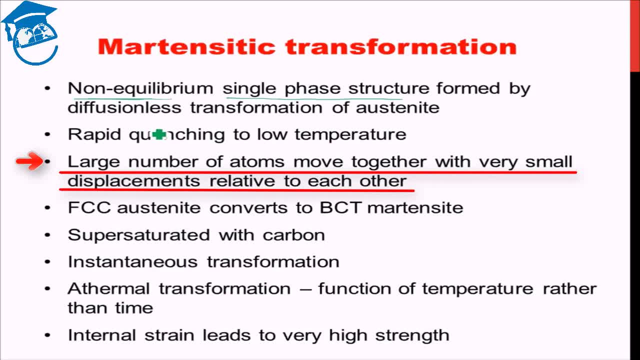 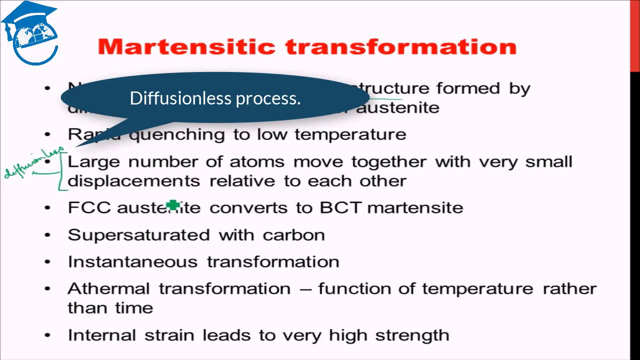 really do not require diffusional processes to be activated: Small distance movement by large number of atoms together relative to each other. that leads to martensitic transformation. Therefore, this is a diffusion-less process. What is happening during martensitic formation? As I said, 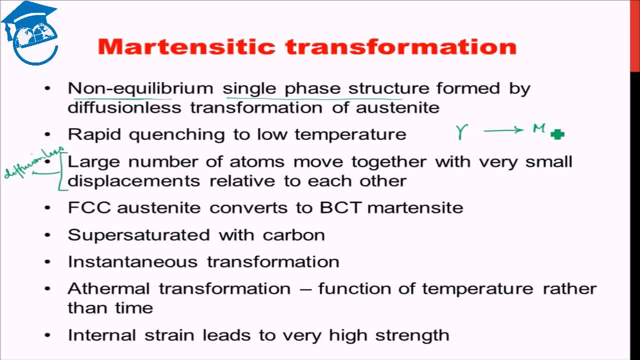 basically, austenite is getting converted to martensite. Now, what is austenite? Austenite is face-centered cubic structure, whereas martensite is body-centered tetragonal BCT. BCT structure is something in which one of the axis is larger than other two axis. So basically, 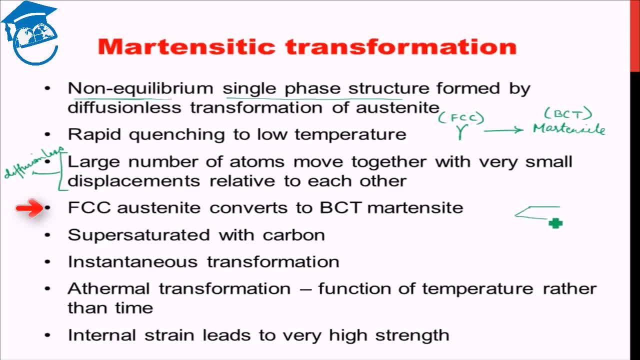 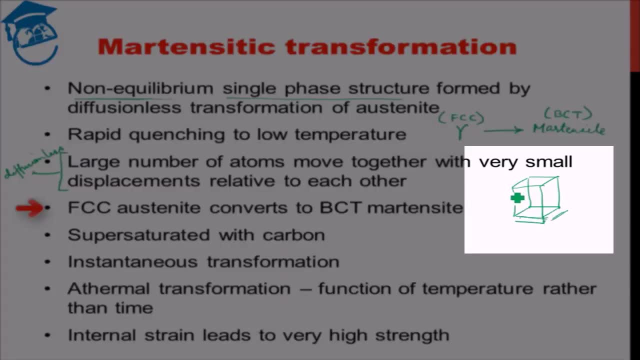 we have a cube, a slightly elongated cube. So it's not a cube, rather a cuboid, but the elongation is very less. These two axis are of equal length. This axis, if this is a, this is approximately point zero, four a around. it actually depends on how much amount of carbon is. 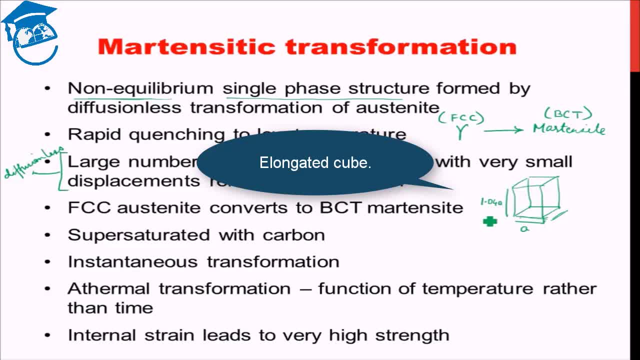 there in the system that will decide this length, but it's approximately till four percent larger in dimension. this dimension now, this BCT martensite, is actually a super saturated solution. it is super saturated with carbon. that is due to the rapid quenching. carbon did not get time to escape out, it could not. 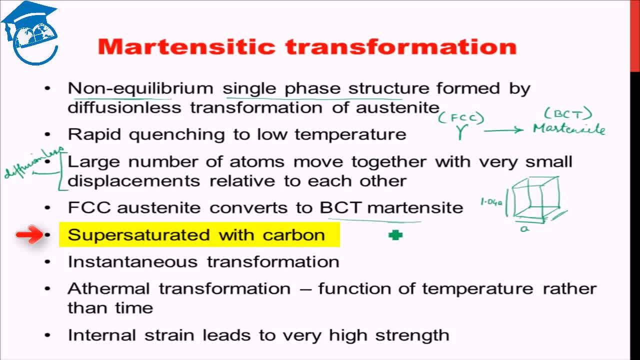 diffuse out of the material and attain the equilibrium state, rather the carbons somehow accommodated within the material, thereby forming the BCT structure, which is super saturated with carbon. and this super saturated carbon, which are present in the tetrahedron, in the void sites, leads to a lot of internal strain, the super saturation. 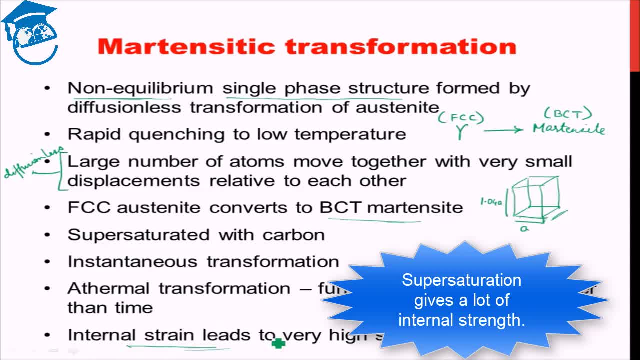 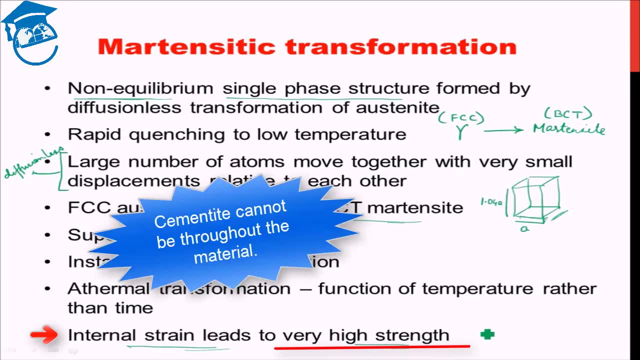 leads to a lot of internal strain, and it is this internal strain which gives martensite a very, very high strength and very, very high hardness. this is the hardest phase that can be made out of steel. cementite is a harder phase, but cementite cannot be throughout the material right. it can be a portion of 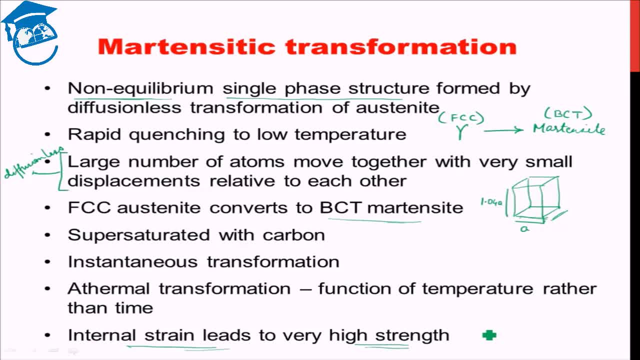 the material. if you want to convert the whole material into one phase, then martensite is the hardest phase possible. hardest, okay, and as I said, that that there is no diffusion involved rather very small amount of displacement which actually takes place at the speed of sound. therefore the transformation is 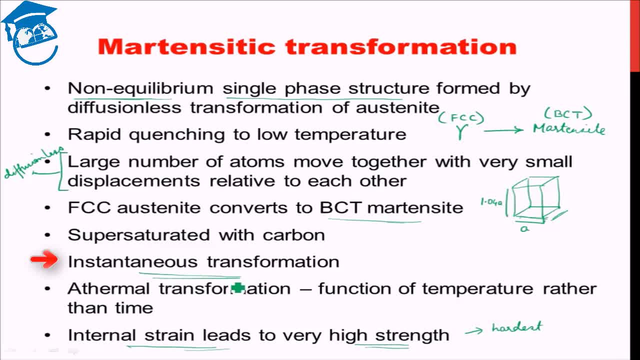 instantaneous transformation. it occurs at the speed of sound. instantaneously the austenite converts itself to martensite and this process- not diffusion driven thereby- it is not time dependent. rather it is a thermal process, that is, it depends on the temperature. the amount of martensite formed during the process is a 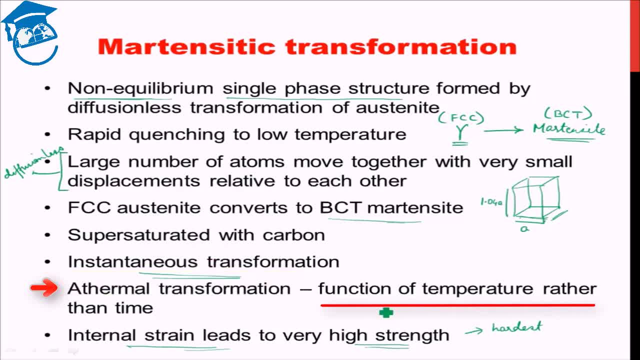 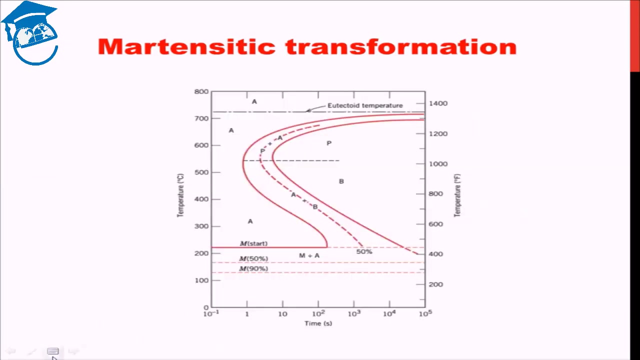 function of temperature. lower the temperature, more is the drive or more is the effect of a, the quenching. lower you go that, go in the temperature, more is the amount of super saturation and larger amount of martensite is formed out of the austenite. okay, this idea we will see in the TTT curve, if you remember from the. 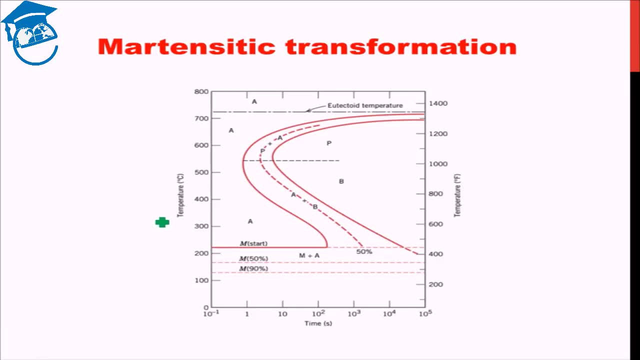 previous lecture I showed you the curve. in the CCT curve also we had these things: M start, M 50%, M 90%. this is the pearlite start, pearlite finish. bainite start, bainite finish. now suppose that you take the material and heat it to the 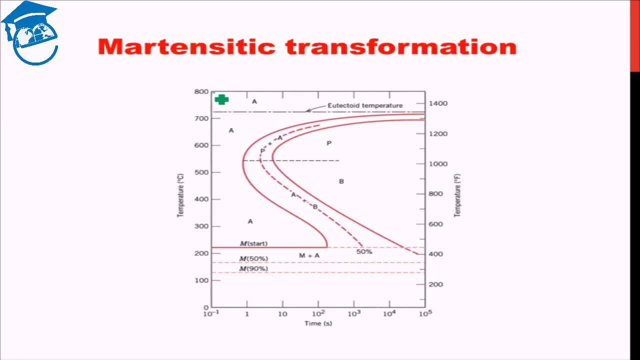 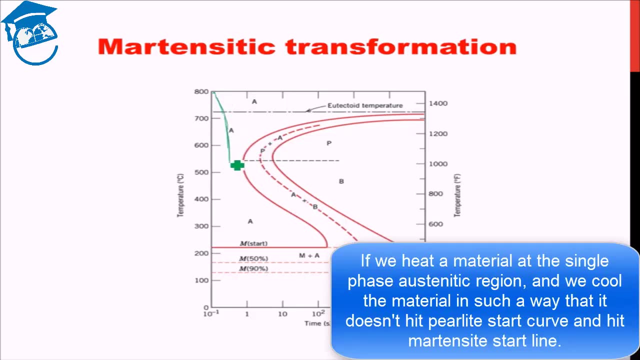 single phase austenitic region and you cool the material in such a way that it does not hit the pearlite start curve, rather it keeps cooling, it is quenched and it hits the martensite start curve. Martin, start start line: when you hit the martensite start line, then martensite 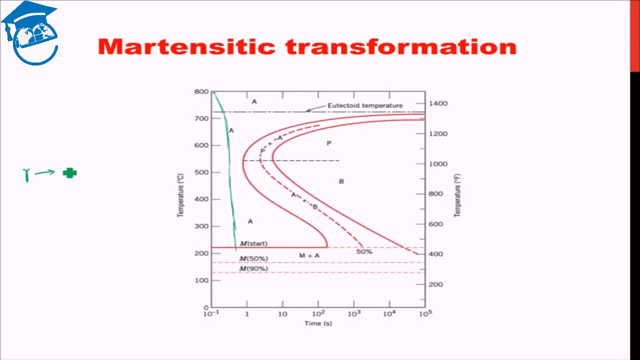 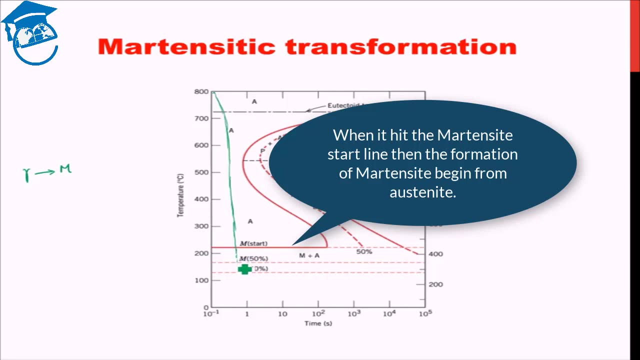 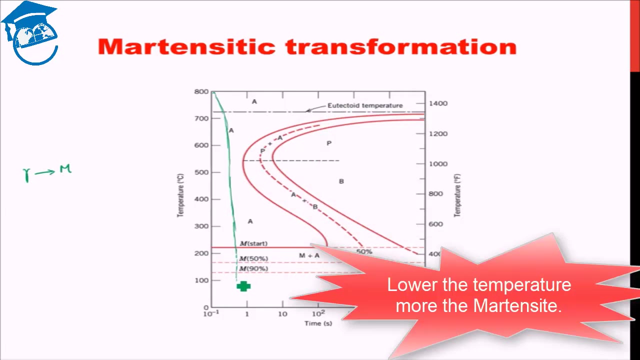 starts to form from the austenite. austenite gives rise to martensite. the lower the material goes at in temperature, the lower it is cooled to, more the is the amount of martensite formed. further lower, further higher amount of martensite form. So basically, during martensitic transformation, what is happening? 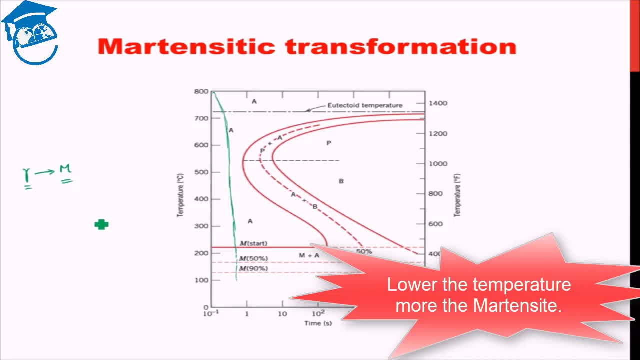 is austenite is getting converted to martensite, but at any temperature you are not really reaching 100 percent martensite. Maybe at room temperature, at 25 degree Celsius, maybe you have M99 percent. maybe at minus 50 degree Celsius you have M99.95 percent, but there is no martensite. finish line as 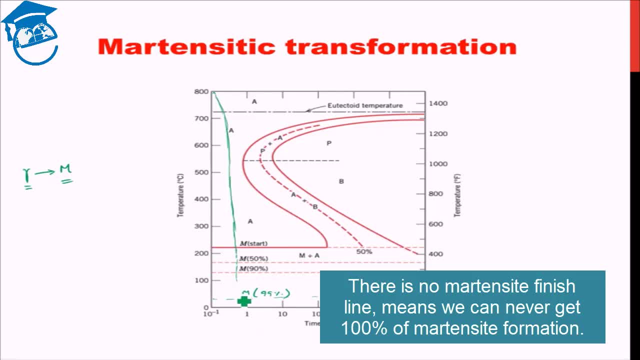 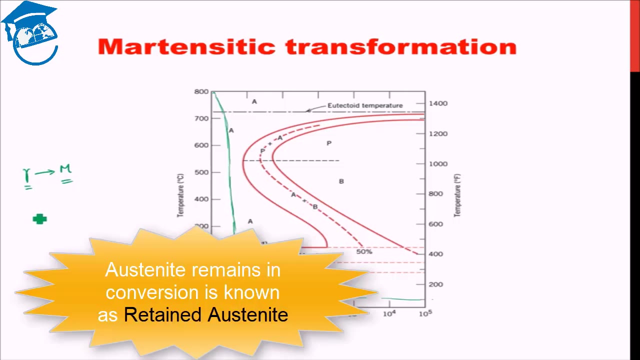 such. So, at any condition, you have austenite converted to martensite, which is a very, very hard phase, as we discussed, but there is some amount of austenite remaining and that austenite is termed austenite As retained austenite. this retained austenite can be useful or harmful, depending on the application. 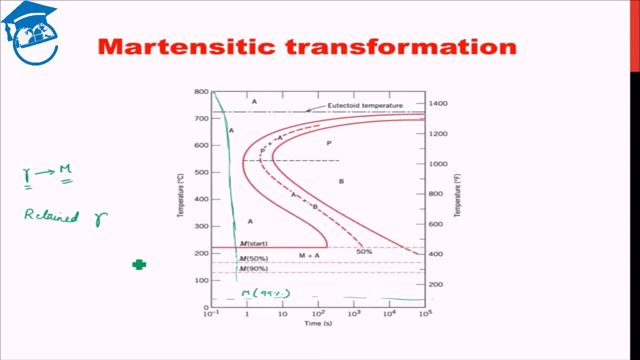 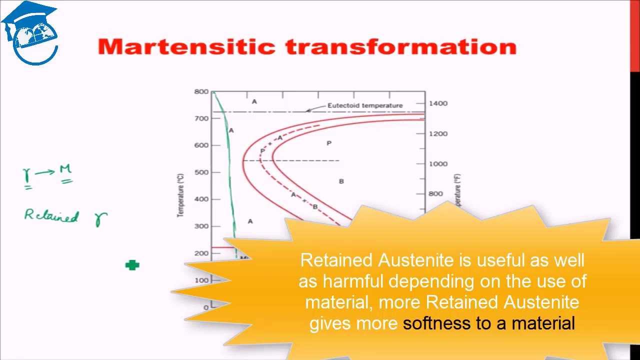 it is put to. Retained austenite is itself a much softer phase than martensite. So if our main criteria is to have a material which has very high wear resistance or very high hardness, then having retained austenite in high percentage can be very 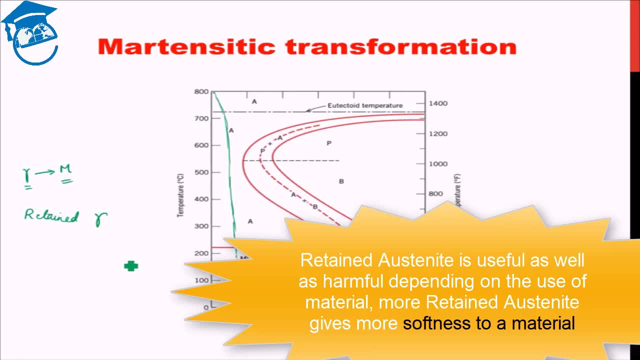 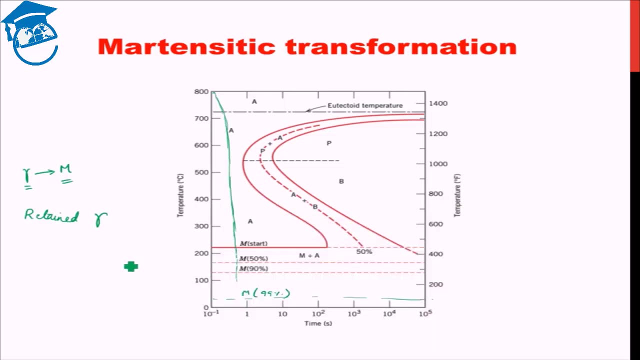 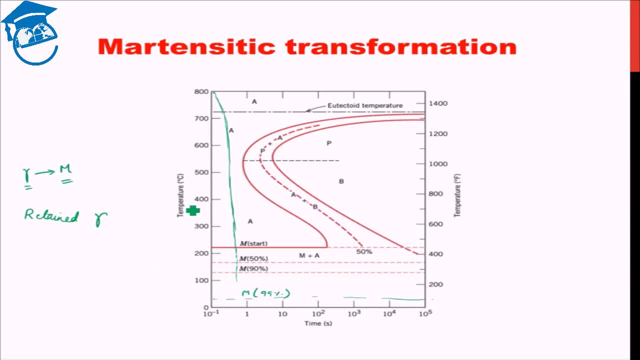 idea which I discussed previously about the shifting of the pearlite start, pearlite finish curves on alloying. similarly, the martensite start and different martensite percentage lines also shift either upwards or downward depending on what alloying element is present and in what percentage that alloying element is present. So there will be different curves for martensite. 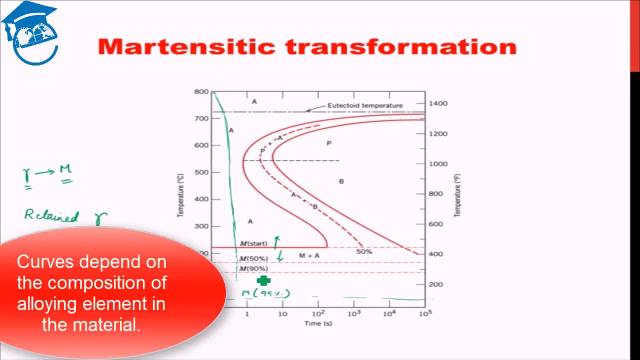 start and martensite, 90%, depending on what is the composition of the material involved. Okay, Now what is the slope of the material? The slowest rate of cooling which will give you martensite. The slowest rate of cooling which will. 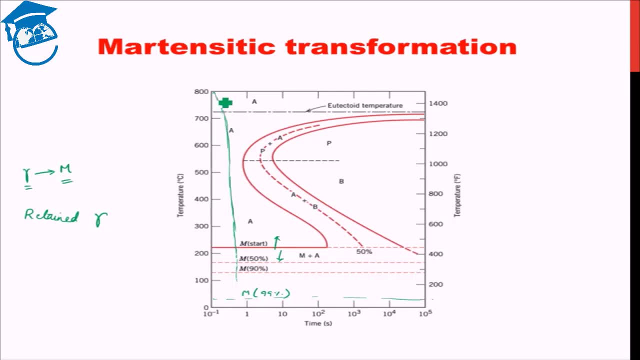 give martensite is the rate where we just avoid the nose. We just avoid the nose, then we are able to plunge into the martensite region. But if we go through the nose then we won't be able to get hundred percent martensite or a very high. 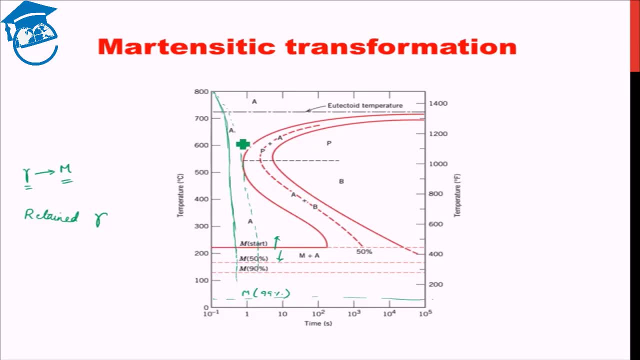 percentage, martensite will also end up getting some pearlite in that system, Right? So this gives you an idea about how martensite is formed. Martensite is basically formed by rapid quenching, rapid cooling of austenitic material. 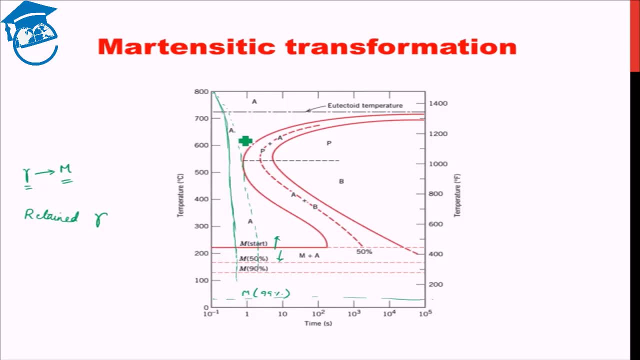 How much martensite is formed depends on the final quenching temperature. how cool you are going? Now let us see Some Some phase transformation scenarios. Suppose I use this cooling curve, Then I get hundred percent pearlite Right now. 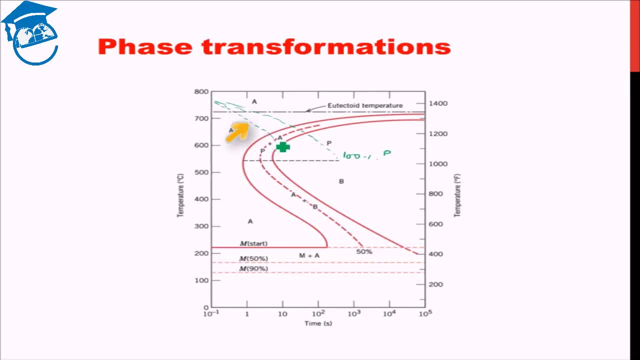 Let's suppose I use this cooling curve and then I quench it. Then I quench it. Then what will happen here? I will form almost 50 percent pearlite, but the rest of the pearlite now, Now rest of the austenite, will now convert to martensite. 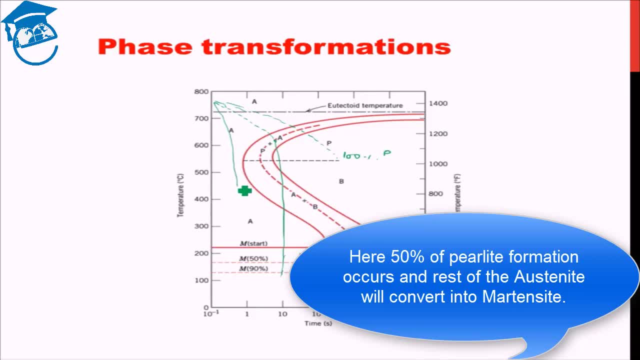 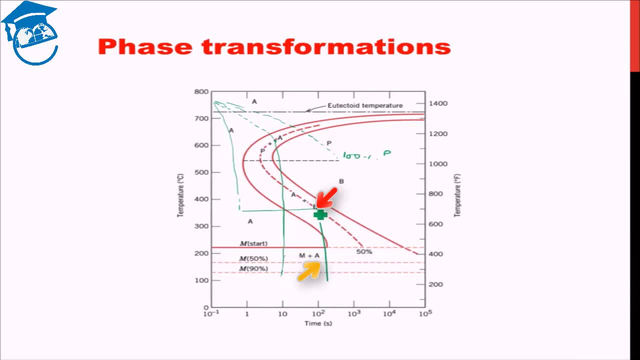 Okay, Similarly, suppose we go here, we go into the bainitic region and then we quench it. What will happen? We'll form certain amount of bainite out of the austenite and the remaining austenite, when we quench it, will form martensite. 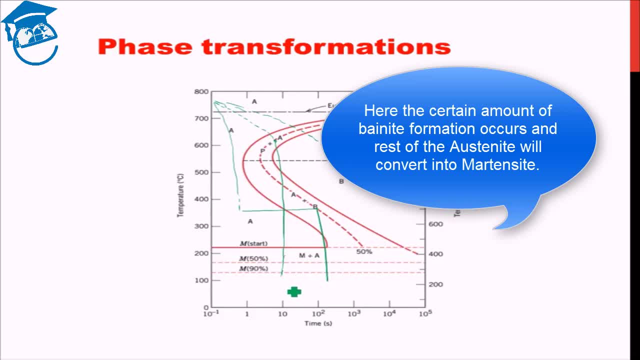 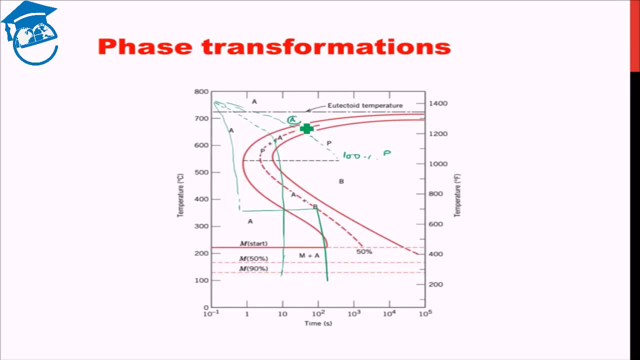 And in all the cases when there is martensite produced there will be some amount of retained austenite. So what are the phases? again, In case A we had 100% pearlite. In case B we'll have around 50% pearlite plus martensite, plus retained austenite. 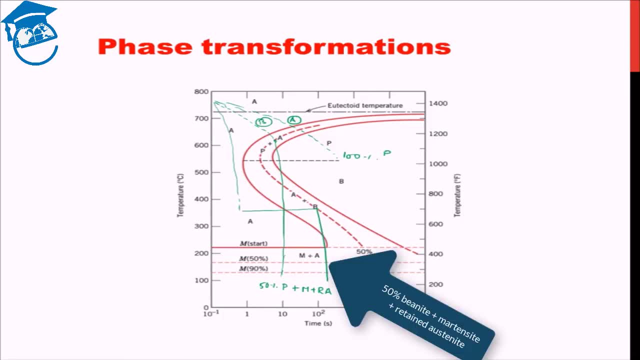 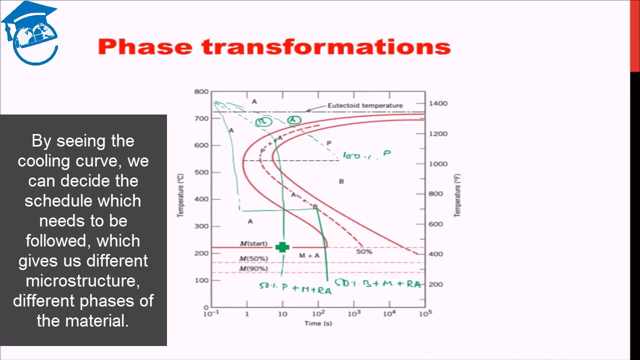 In this case we'll have almost 50% bainite plus martensite, plus retained austenite. So by seeing the cooling curve and we can decide the schedule Which needs to be followed, and that schedule will give us different microstructure will.